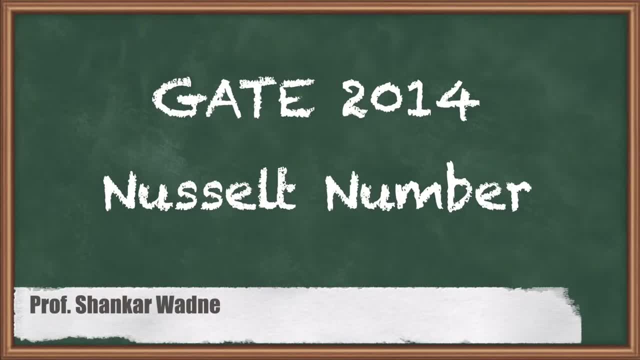 Hello, my dear students, in this lecture we are going to see one previous year gate numerical. This question was asked in gate 2014 for two marks in set 1.. Basically, this question is based on finding nascent number with the help of convection heat transfer. 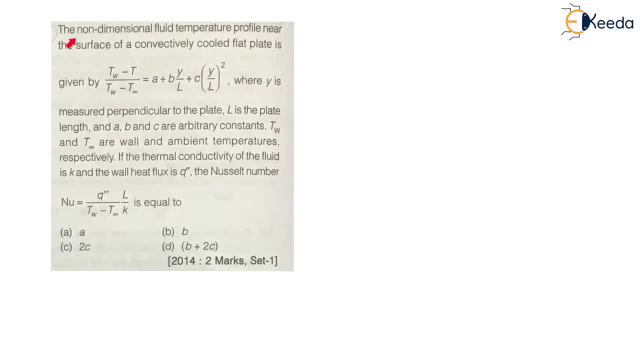 So let us understand the question. The question is: The non-dimensional fluid temperature profile near a surface of convectively cooled flat plate is given by Now. here the temperature profile is given. Can you say here the temperature profile is a function of y. 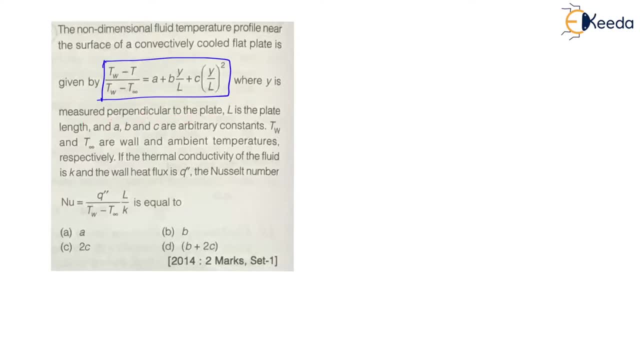 Where y is a measured perpendicular to the plate. Let us say there is a plate. If I draw one plate, For this plate The perpendicular direction is y And, my dear students Here, generally the thermal boundary layer forms like this: Let us draw here thermal boundary layer. 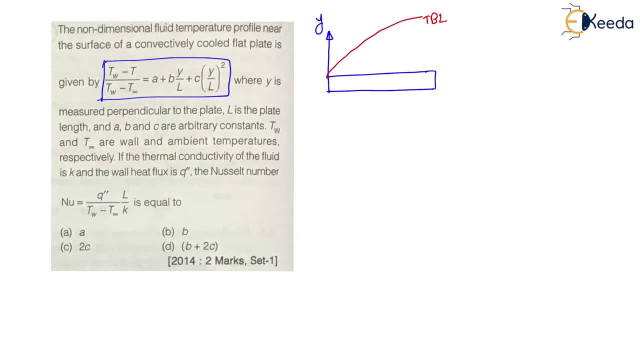 Thermal boundary layer is formed like this Thermal boundary layer And, my dear students, in this thermal boundary layer This temperature profile is given. Therefore, here the wall temperature will be, Here they have mentioned further. Let us say, measured perpendicular, Where y is measured perpendicular to the plate. 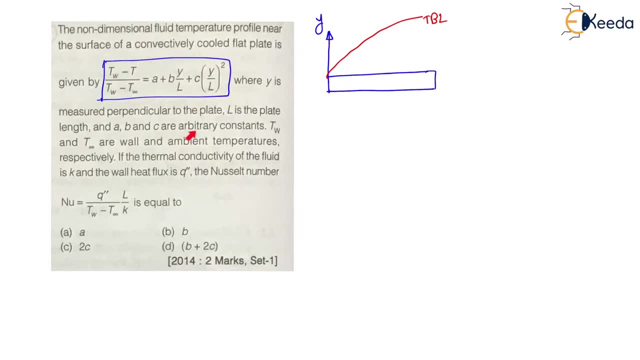 L is the plate length. A, B, C are arbitrary constants. T- wall and T- infinity are wall and ambient temperatures respectively. Now here, my dear students, Length of plate is given, L For this plate length is L. A, B, C are constants. 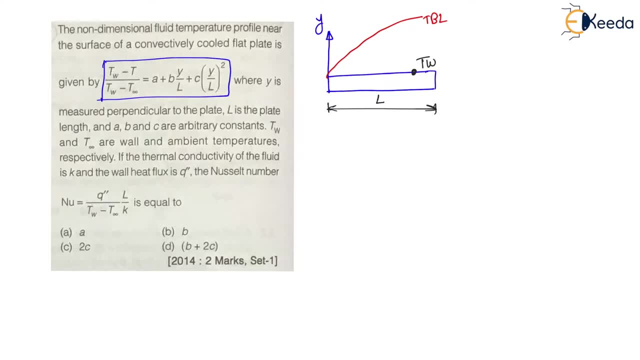 And this surface temperature, or wall temperature, is T, w, And surrounding fluid temperature is T, infinity. And in this thermal boundary layer, The temperature is T. The temperature is T And, my dear students, this temperature profile is given here With respect to L, A, B, C and Y. 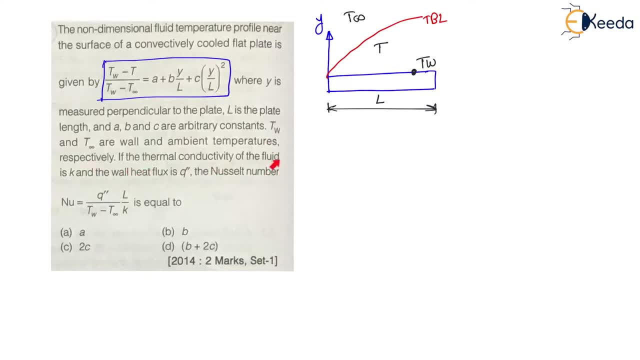 Then if the thermal conductivity of the fluid is K And wall heat flux is Q, double dot The Nusselt number NU is given. Now, here, Nusselt number is given. My dear students, they have given the thermal conductivity of fluid, not plate. 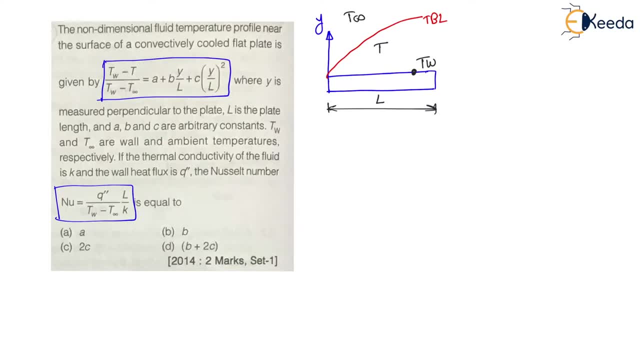 Now, here, there will be a fluid. Let us understand. Let us say: there will be a fluid like this: If I draw one fluid In this boundary, there will be a fluid. This will be the fluid Right And, my dear students, for this fluid. 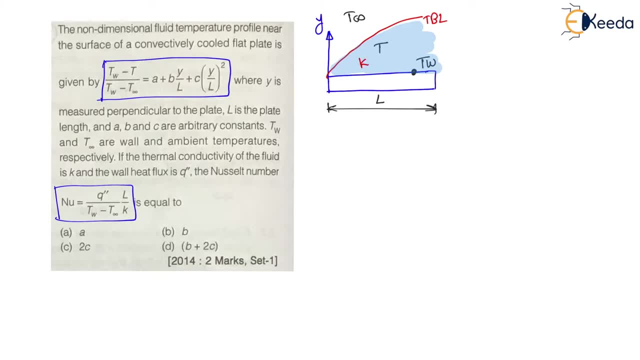 Here they have given thermal conductivity K Right. So here again Nusselt number relation is given, That is, heat flux divided by temperature of wall, minus T, infinity L by K. Now this Nusselt number we have to find In terms of this A, B, C, arbitrary constants. 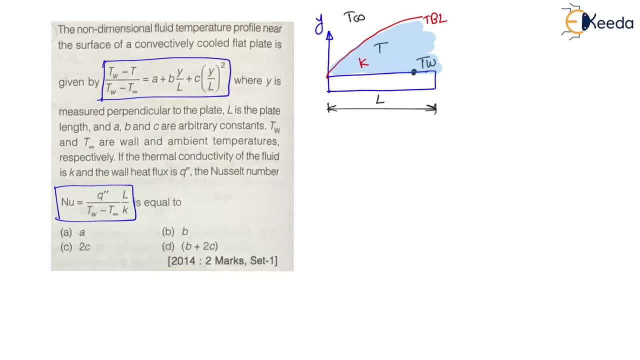 Now let us understand here the mechanism of heat flux. Right, My dear students, let us assume the wall temperature is more than fluid temperature. Here I am assuming wall temperature is more than fluid temperature, T infinity. Therefore the heat will flow from plate to the surrounding. 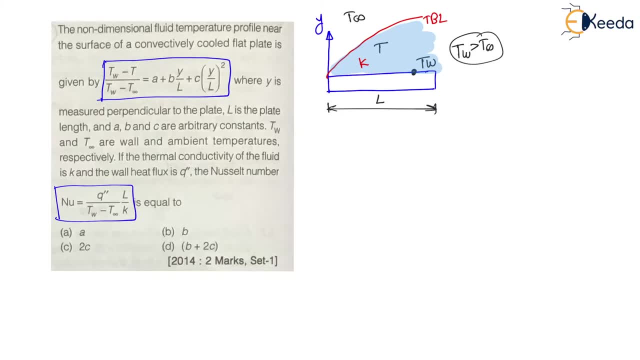 Right Now, the first layer of this fluid in contact with plate, I will say the first layer of this fluid in contact with this plate, there will be a conduction. I can say, on this first layer there will be a conduction: heat transfer. 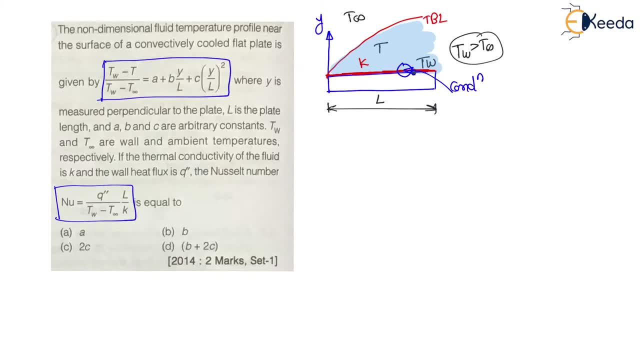 Right And my dear students, again, between this plate and surrounding fluid there will be a convection. Later there will be a convection. heat transfer. Right And my dear students, for steady state condition. whatever may be this conduction, heat transfer. 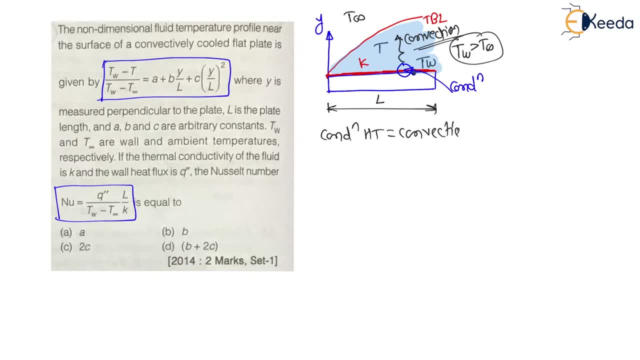 is always equal to convection heat transfer. Convection heat transfer For steady state condition. now, whatever may be, the heat conducted through this first layer of fluid is again convicted to the surrounding fluid. Right Now, this heat conducted or heat convicted, which is nothing but Q, is given by as per. 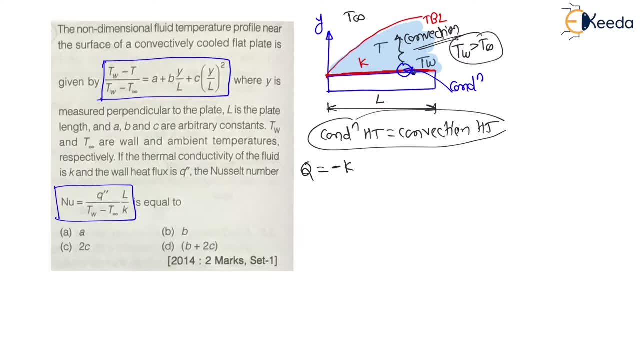 Fourier law of conduction, heat conducted is given by minus KA dT by dx. This is the heat conducted. And heat convicted, as per Newton's law of cooling is given by HA T wall minus T infinity. Right Now, this is a Fourier law of conduction, minus KA dT by dx. 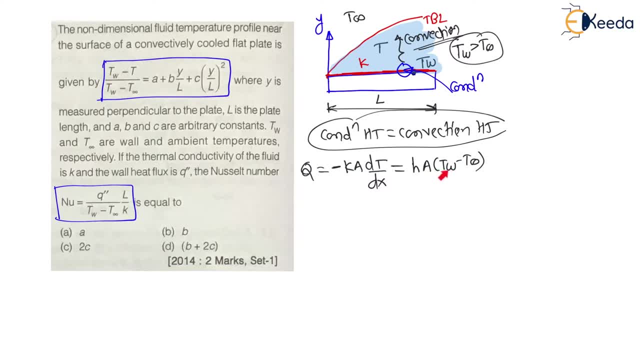 And this is a Newton's law of convection, that is HA T wall minus T, infinity, Right. But they have given heat flux Q double dot. Therefore, my dear students, this Q double dot is nothing but Q divided by area heat. 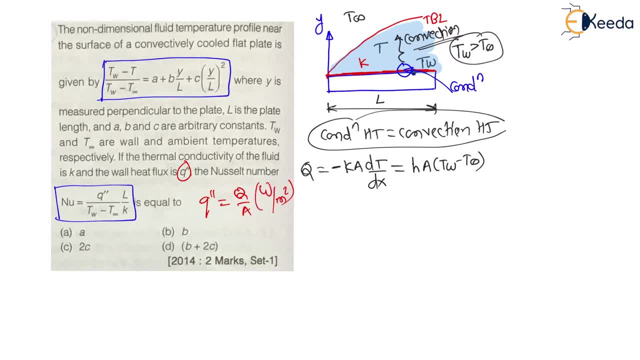 flux, that is Watt per meter square. Let us write this Q double dot as heat flux. Therefore here can I say: Q divided by area, which is Q double dot, is equal to divided both side by area minus KA, dT, by dx, which is equal to EH T wall minus T infinity. 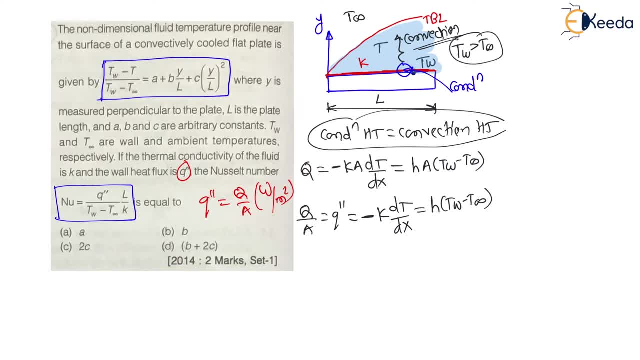 Right, This will be the heat flux. Now, My dear students here, the Nusselt number relation. we know that it is HL divided by KA of fluid. Now can I say from this relation: let us equate Q double dot with H, T wall minus T, infinity. 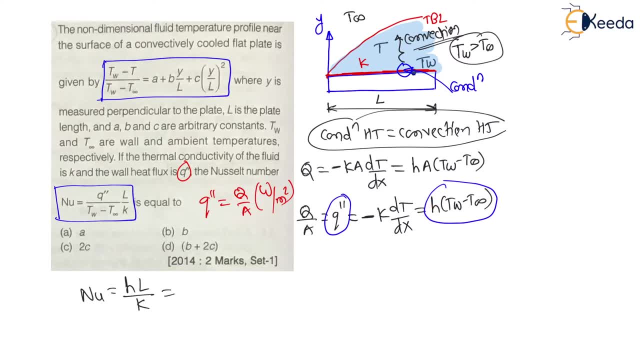 Right. Can I say from this: this H will be equal to Q double dot divided by T wall minus T infinity. Therefore, this H is heat flux divided by T wall minus T infinity into L divided by KA. Same relation they have given here. 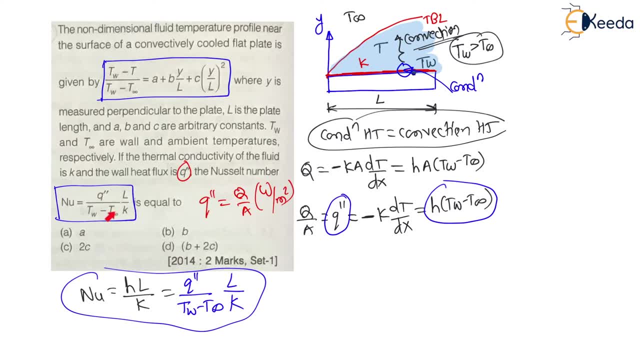 There is absolutely no need to provide this relation because we know that the EH is nothing but heat flux divided by temperature difference. Right Heat flux divided by temperature difference is this convective heat transfer constant, EH and Nusselt number is HL divided by KA. 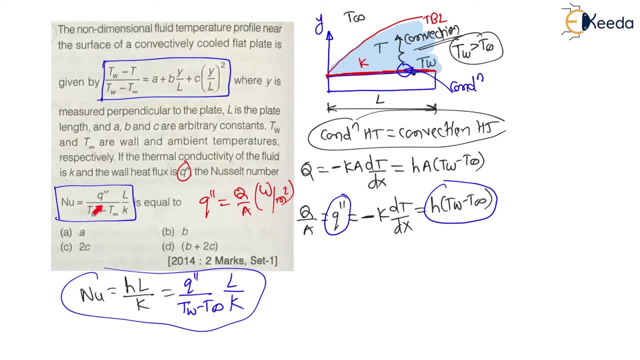 But anyhow, they have given the relation, Let us use this relation Right. So if I want to find Nusselt number, I have to find heat flux, and to find heat flux, as here, temperature profile is given. Therefore, if I differentiate this temperature profile, I will get temperature gradient dT. 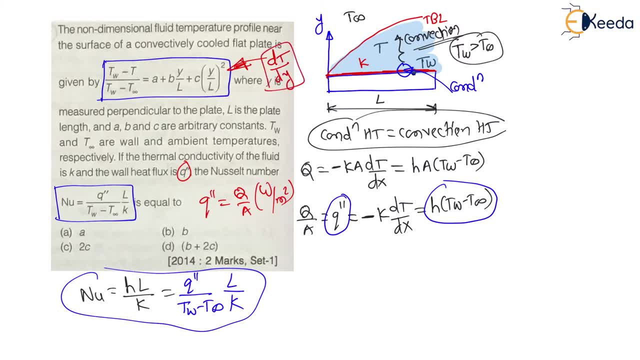 by dx or dT by dy, here with respect to y Right As it is with respect to y. therefore, instead of here x, let us write here y Right, Here y Right, Because it is along y direction. If it is along x direction, we are writing dT by dx. 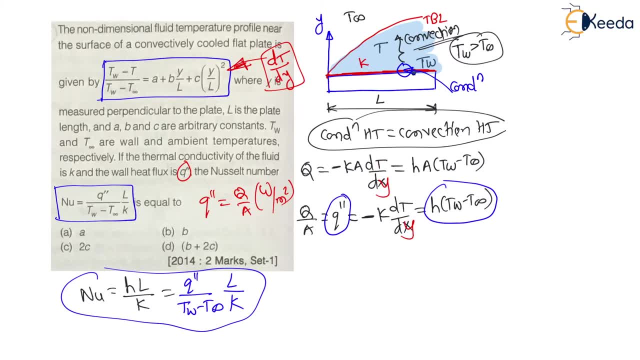 If it is along y direction, we are writing dT by dy Now. so if I differentiate this equation, I will get temperature gradient dT by dy, Right, And if I get temperature gradient dT by dy, then I can find heat flux. and let us put: 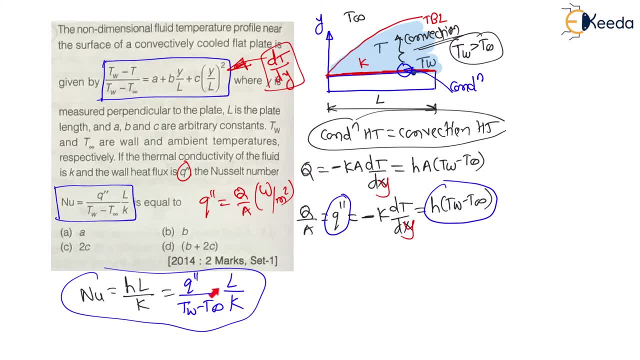 this heat flux, in this Nusselt formula, Nusselt number, formula Right. So, my dear students, let us find this Nusselt number: q, double dot is equal to minus k, dT by dy. So, to find this Nusselt number, let us find first dT by dy. 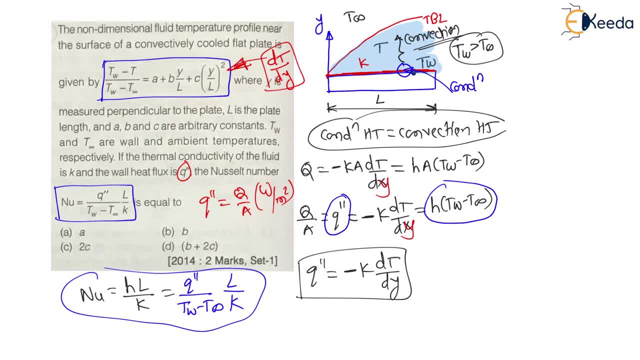 We have temperature profile over here Right Now. let us make a sufficient space for the solution. Now let us find this heat flux first, Right, And then use this heat flux in Nusselt number formula. Now, my dear students, therefore, can I say this heat flux? therefore, here this heat flux. 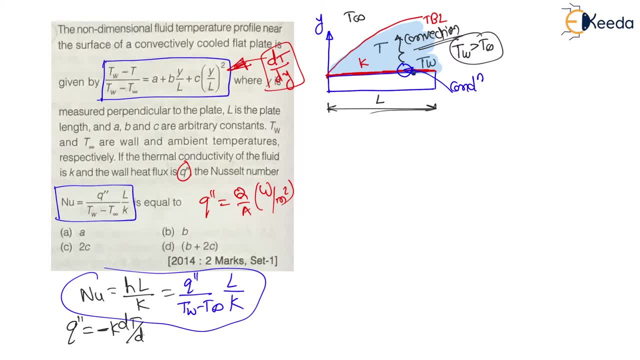 q, double dot is equal to minus k dT by dy. So here again our new target is to find dT by dy. Now here temperature profile is given. Let us use this temperature profile: Wall temperature minus temperature divided by wall temperature minus T, infinity is equal. 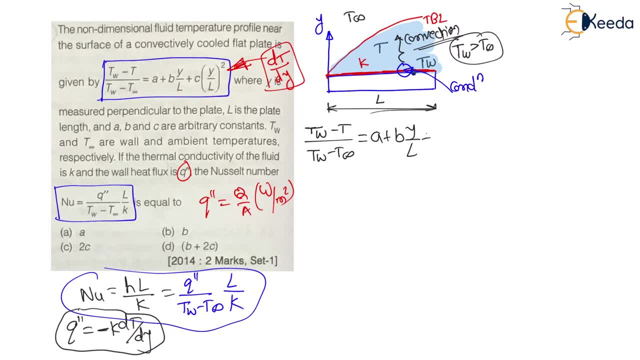 to a plus b, y by l plus c, y by l whole square. Right Now, here let us take this T wall minus T infinity on the right side, Because this wall temperature and surrounding fluid temperature is always constant. only variable is temperature with respect to y. 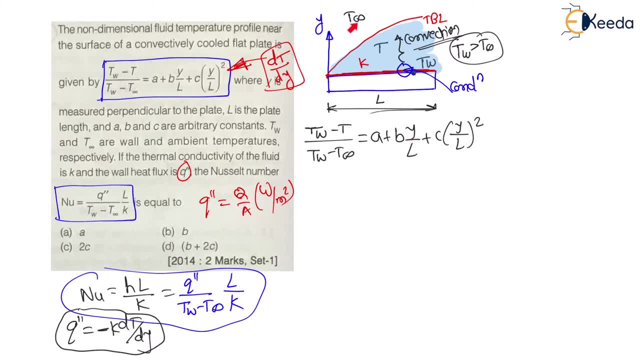 Wall temperature for steady state condition and fluid temperature for steady state condition is always constant. Therefore the equation becomes: T wall minus T is equal to T wall minus T. infinity Right Into a plus b, y. by l plus c, y square by l square. 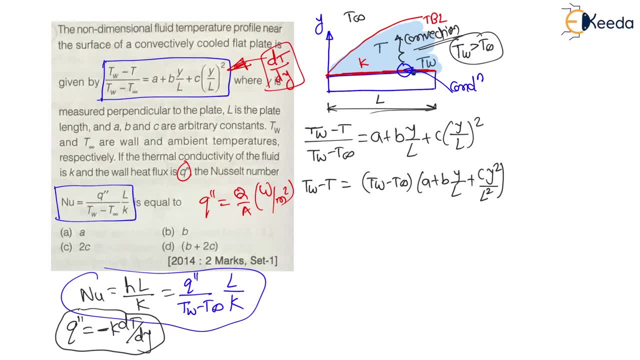 If I square it separately, y square by l square. Right Now, my dear students, let us differentiate this equation. If I differentiate this equation with respect to y, then here therefore, d dT of, we can say d dy of T, wall minus T. 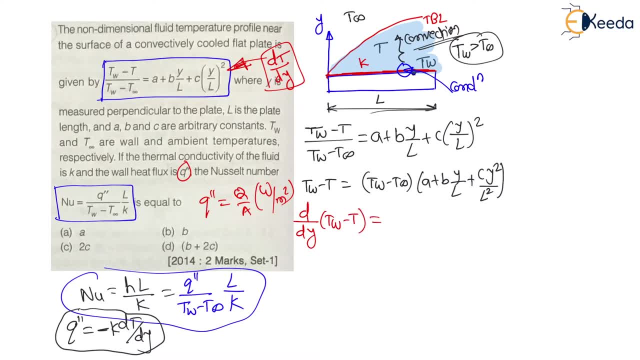 d dy of T wall minus T is equal to y. Now let us differentiate. Can I say it is equal to d dy of T wall minus T? T wall is a constant. Derivative of constant is 0. It will become 0 minus here. dT by dy. 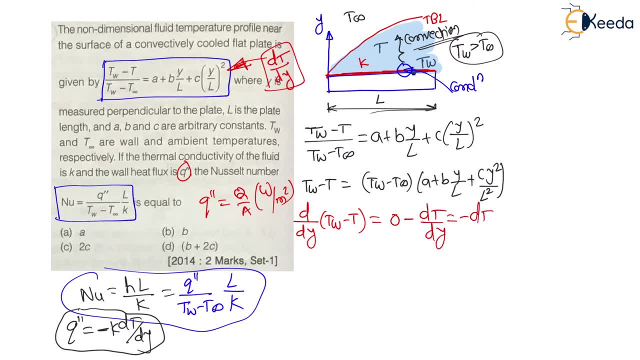 Therefore it will be minus dT by dy. From this we will get value of minus dT by dy. So let us differentiate this equation. Therefore can I say here: minus dT by dy, minus dT by dy, is equal to. 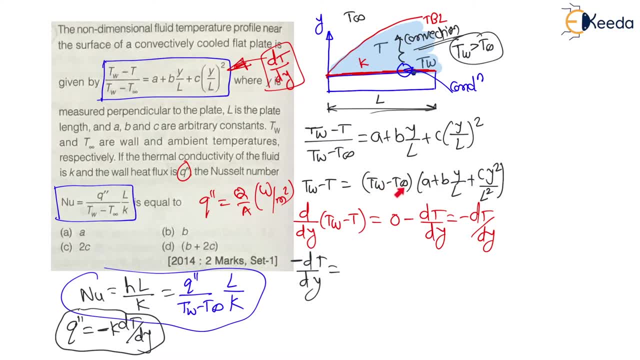 Now consider derivative of this. Now here, T wall minus T infinity is constant. Therefore, let us use this constant T wall minus T infinity constant Right Now. differentiate this expression with respect to y. Now derivative of a is 0, because a is a constant. 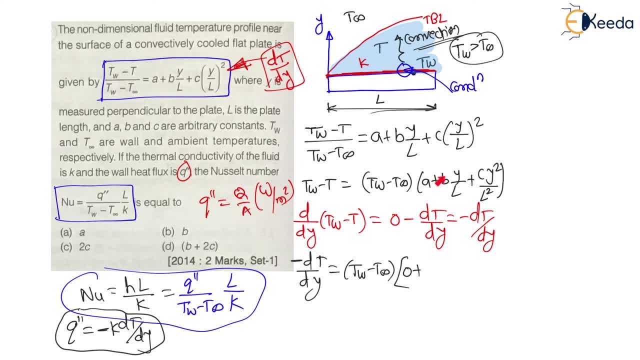 Therefore 0 plus Now, here b by l, again constant. Therefore, derivative of y is 1.. Therefore, here b by l, plus Again, here c by l, square is constant And derivative of y square is 2y. 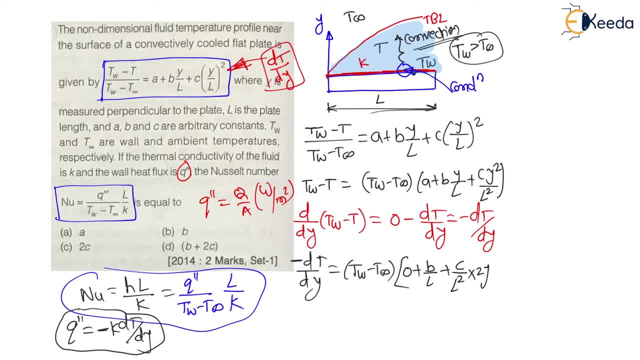 Therefore, here, t by l square into 2y Right, This will be the expression. Therefore, my dear students, minus dT by dy is equal to T wall, minus T infinity into d. by l plus 2tl square into y: 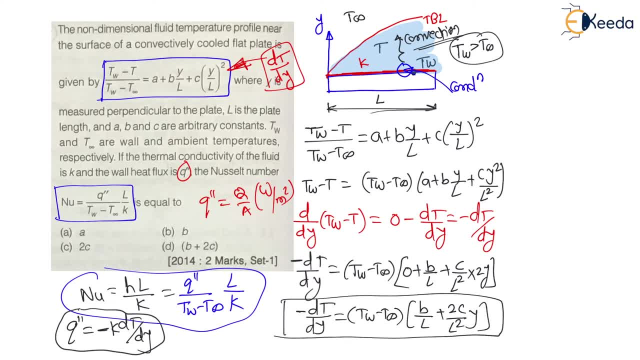 This will be our expression: Right For temperature gradient, Right Now. let us observe the diagram. Now, my dear students, At what location there will be a conduction and at what location there will be a convection? Just now, at the start, I have explained this phenomenon. 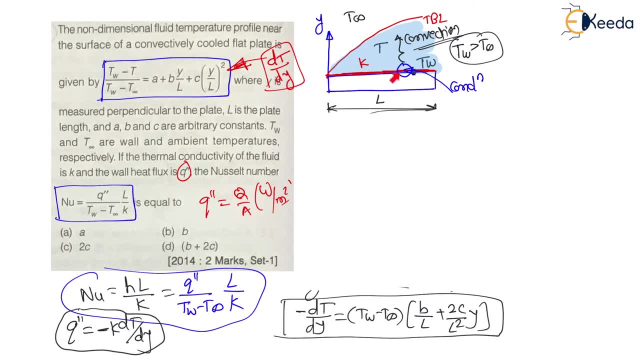 See on this plate the first layer of fluid in contact with plate. there will be a conduction Right Now. therefore, this first layer of fluid in contact with plate will be at a distance. y is equal to 0. Right. 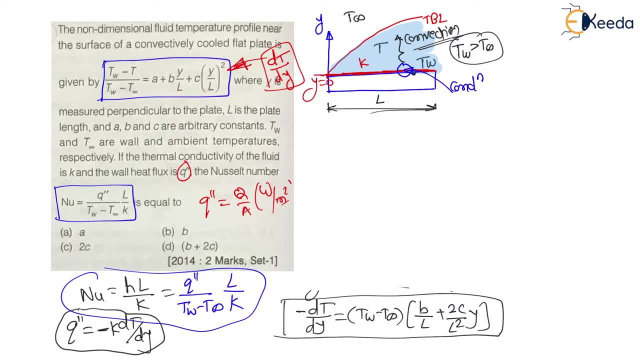 Therefore, whenever y is equal to 0, there is a conduction, And as y is increasing, if I go away from the plate, there will be a convection Right, And this dT by dy is required in conduction equation. 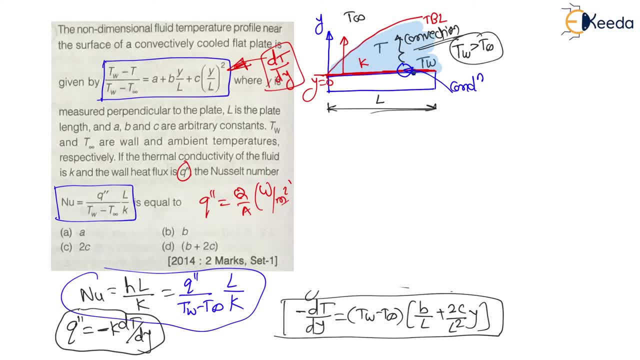 Minus k dT by dy is a conduction equation. Therefore, my dear students, here conduction is at y is equal to 0. Therefore, we can say: whenever y is equal to 0, there is a conduction. Therefore, we can say this: minus dT by dy, whenever y is equal to 0, is equal to. 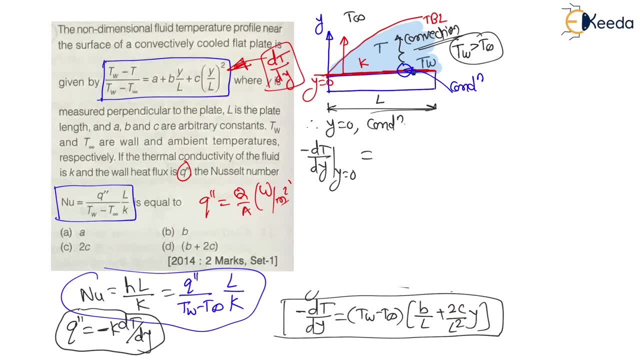 Let us put here: y is equal to 0. Therefore this term will get eliminated. If I put y is equal to 0, this term gets eliminated. Therefore the equation becomes. Therefore the equation becomes T wall minus T infinity into B by L. 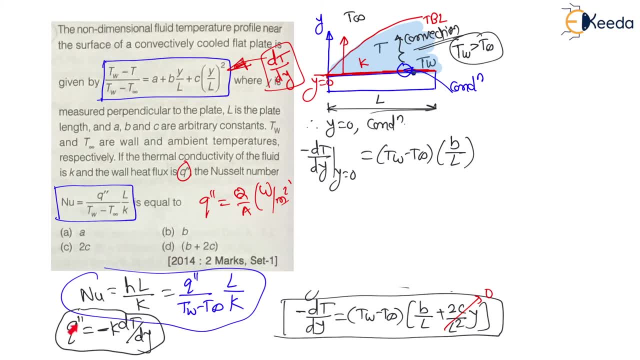 This will be the expression Right Now, my dear students, let us find this Q double dot, That is, heat flux. Now we have this. heat flux is equal to minus kA, minus k, sorry, dT by dy Right.